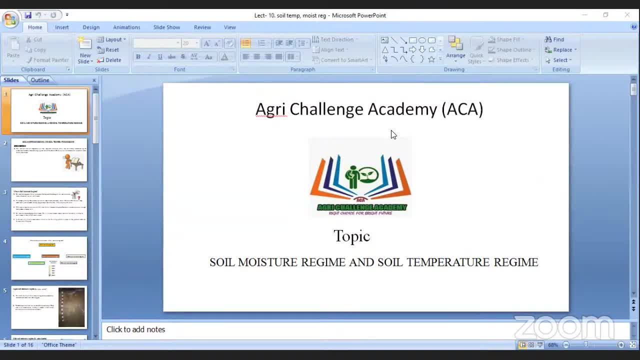 Just to give an example, what you can see, you can use. some particular crop can be grown there. You can give an advice. we can go for this crop, this crop. We can't grow tea crop in southern Andhra Pradesh At the same time. you can't grow some other crops like sorghum, all those things in Uttar Pradesh. 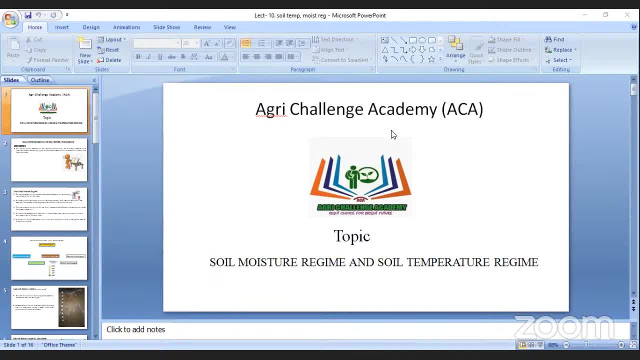 That is very difficult, So that varies. So, for the purpose of classification, For the purpose of classification of the crop cultivations and for the perfect scientific study of particular soils, We are depending upon this soil moisture and temperature regimes. What are those? 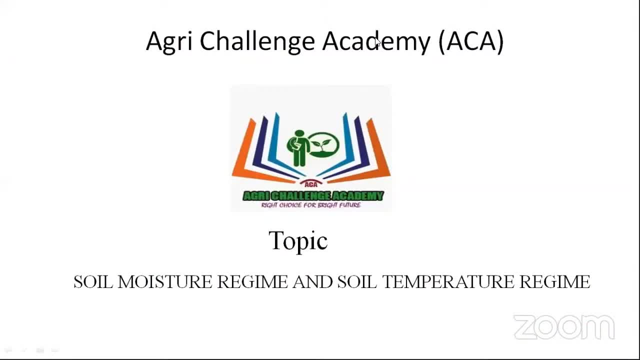 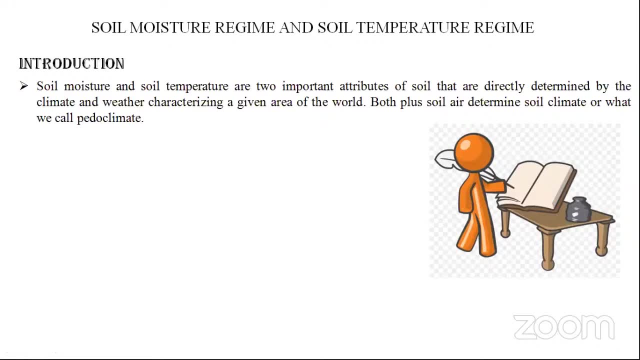 We will see one by one. Is it visible to everyone? Yes, sir, OK, All right students. Introduction. So very first we want to see the introduction of any any lecture. What is the introduction of this soil moisture regime and soil temperature regime? 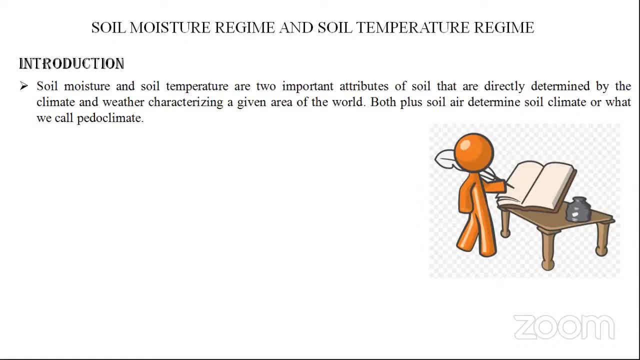 These are the two important attributes. Students, The directly determined. determined by the. What are the factors that directly determine climate and weather? Both have different meaning. Students, If you are interested in meteorology, they will give proper definition about these two. 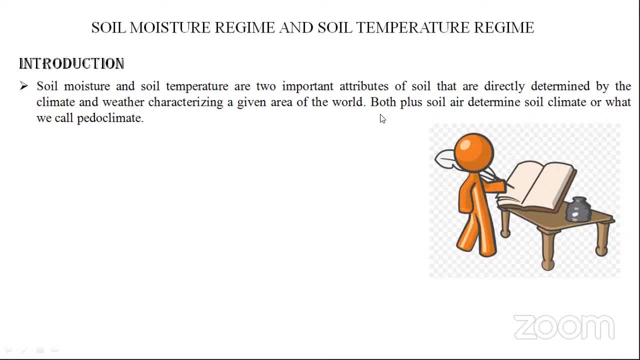 Climate and weathering characteristics given a given area of the world, So a particular particular area. There is this. This climate and weathering will determine the soil moisture and temperature conditions. Both the soil and soil air also will determine by the soil climate, or what called the pseudo climate. 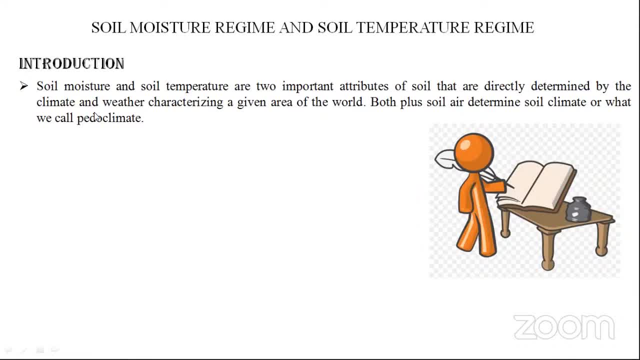 Pseudo climate means it's not a climate, It's climate alike. It's not a real climate, It is a false climate. You know, that particular area of the particular set of soil- We can see this today, This, this, most soil moisture is in and soil temperature is in by the influence by which is determined by the climate and weather conditions. 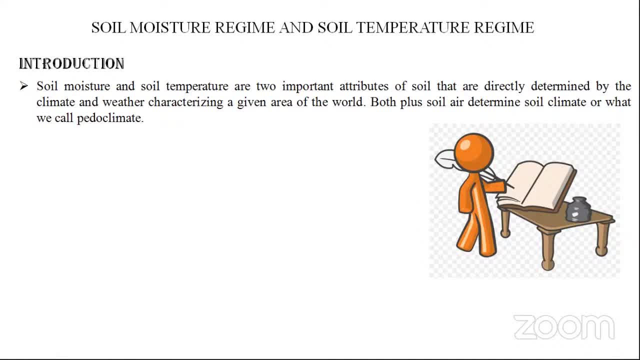 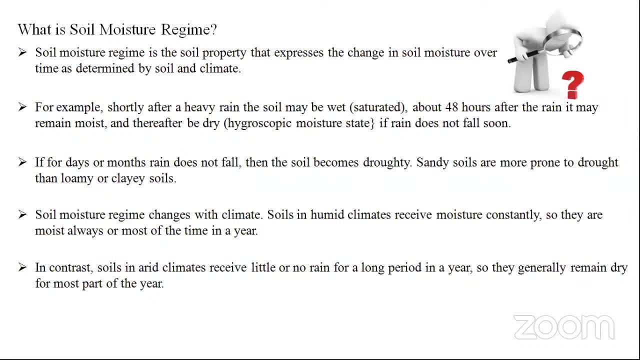 This is. this is a small part of introduction about this. soil moisture and soil temperature is in. Now we will see. sir, What is soil moisture is in. You know, there's nothing but expression of changes in soil moisture. There's nothing but changes in soil moisture. 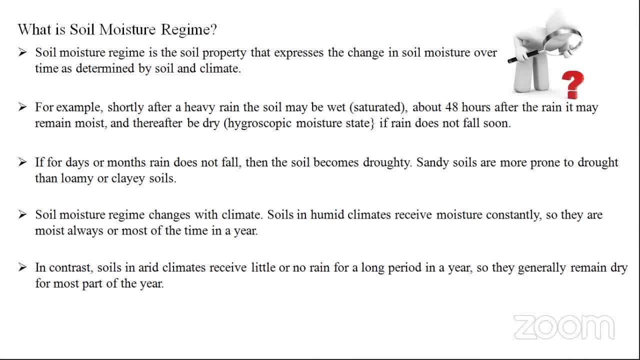 You know, students, In heavy rain, You know, sometimes recently we have experienced, especially in my area, my area, southern coastal Andhra Pradesh, even Hyderabad, those in Telangana, Hyderabad, a part of Chennai, a part of area. 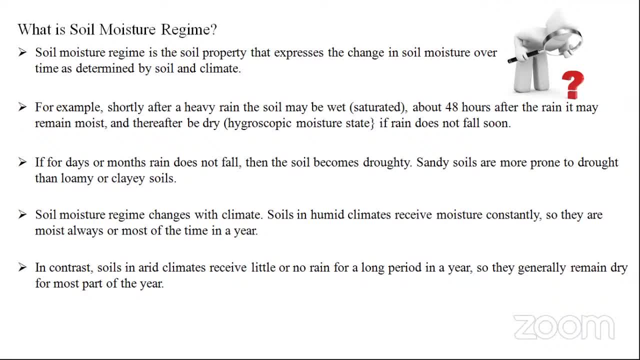 There are heavy rains, are there sometimes, And all the complete soil was completely submerged. The moisture was very heavy. It will deter, So the soil will experience some sort of moisture And that's a situation. at the same time, Students, Any in somewhere in summer season, in the summer season or any any particular weather. 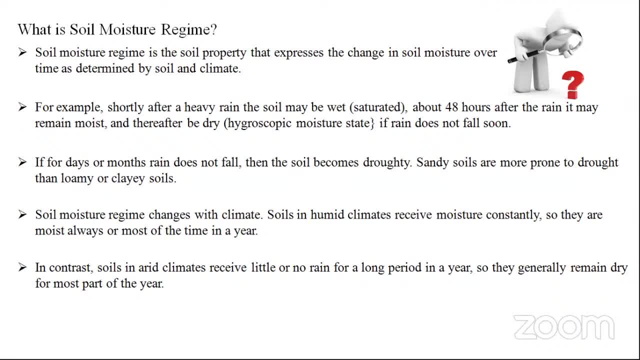 The monsoons was not came, You can see that same solid, completed, dried up at that time Moisturizing will be different. So when the when the rainfall is there, you can see one type of moisture is in when there is no rainfall. 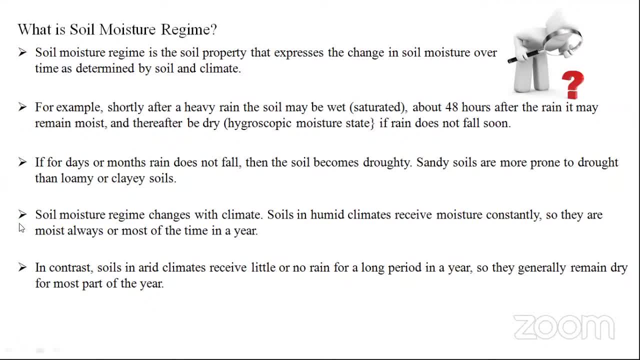 You can see another type of rainfall. So this is what explaining in the in this session, In the second one, In the second: what is that? Shortly you can, shortly after heavy rain, The soil may be wet, Saturated About 48 hours. 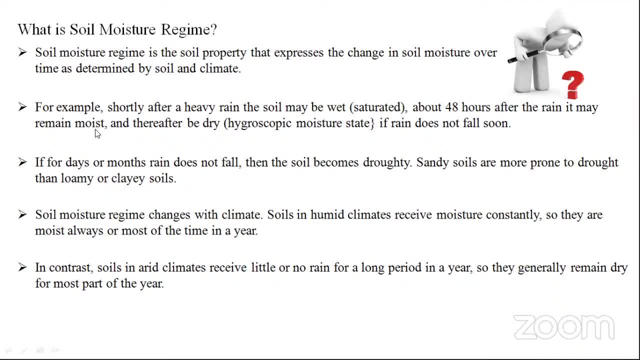 After the rain It may remain moisture. No, After. the complete rain was came after two days, After 48 hours, The soil may become moisture And thereafter by dry. After, after, when the moisture was completely reduced, we can see dry. 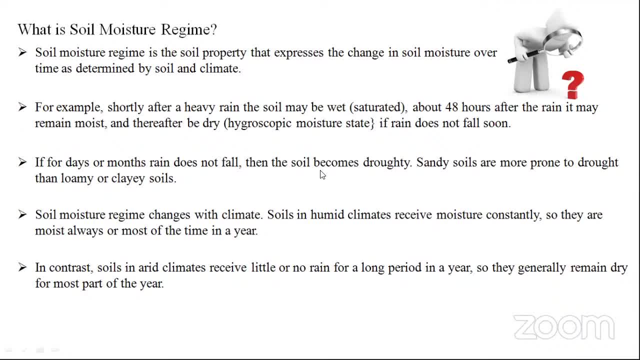 There is hydroscopic, You know, some sort of small moisture will be there. There is one type of machine And if the rain does not fall, what will happen? The complete soil will become drought. There is no rain for months and years. 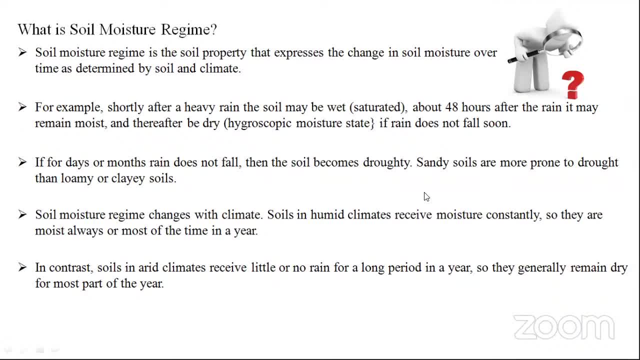 What we can see, that soil become drought, Especially students. Sandy soils are more prone to drought. Students. Sandy soils are highly because very poor structure. Sandy soil, Sandy structure can't hold the water proper. That's where you can see drought conditions. 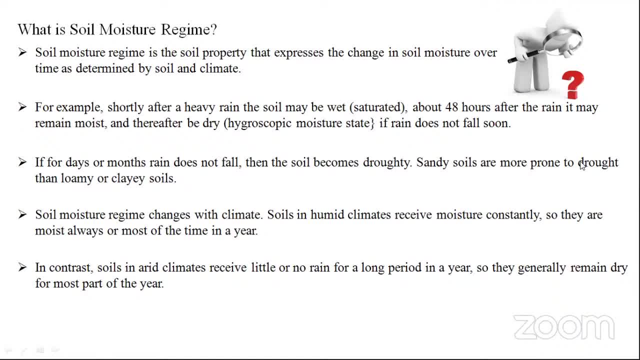 And this has been compared with loamy and clay soils. Clay soils are whole loamy and clay soils are whole moisture. very well, And compared with sandy soils, The same time, Students, The soil moistureism changes with the climatic conditions Completely. 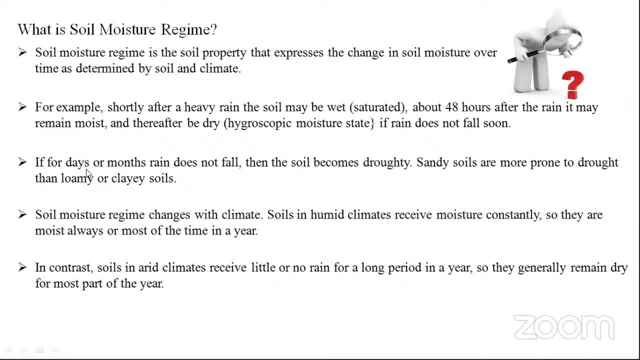 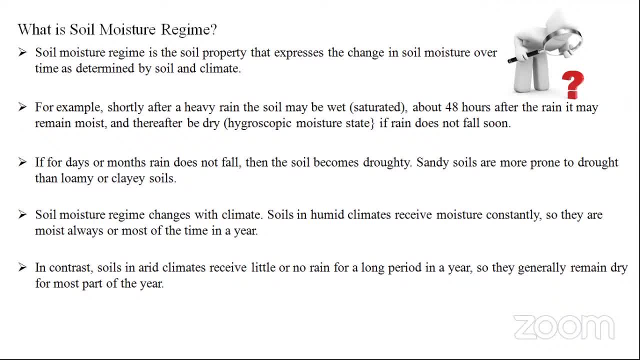 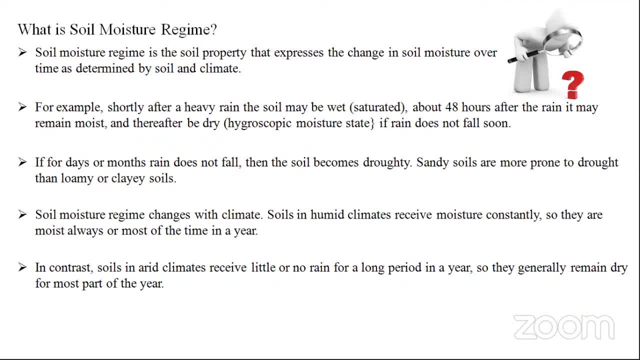 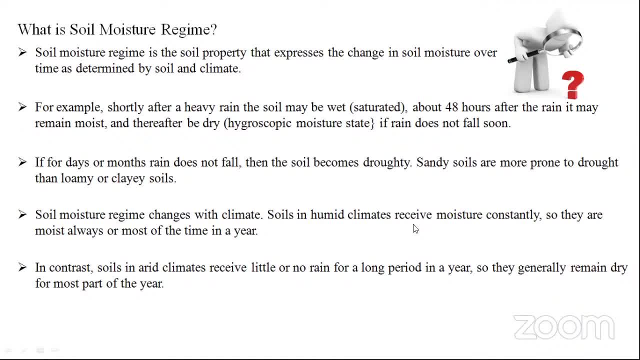 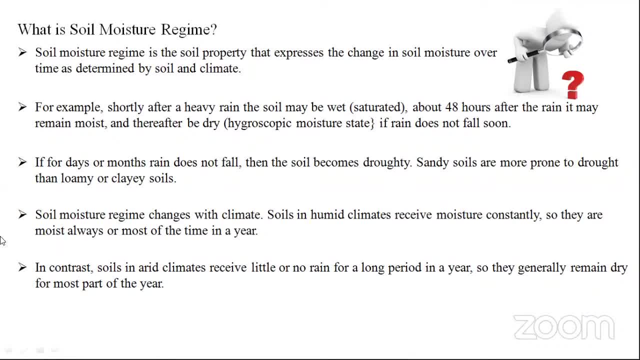 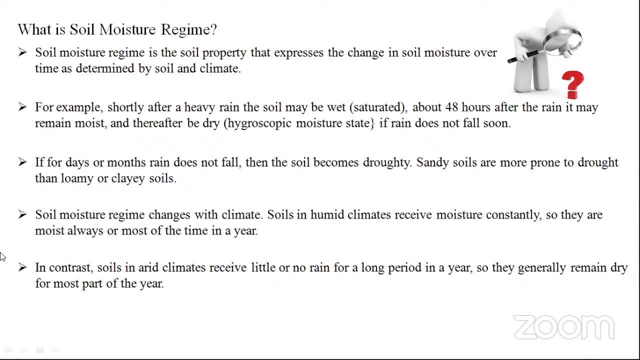 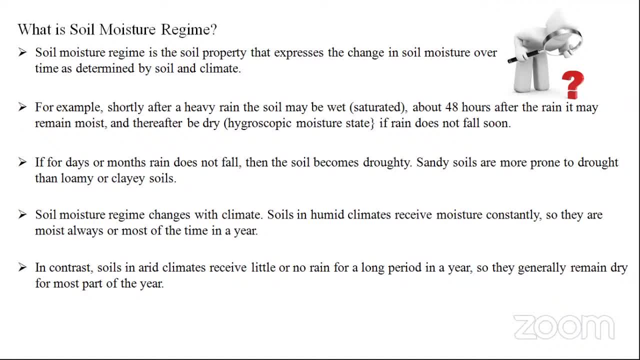 saturated soil, so always complete. saturated water means we have one type of soil moisture regime. if the complete water was drained up and we have some sort of hydroscopic state is there that have one type of moisture regime. and if the soil was completely dried off, nothing is there there. 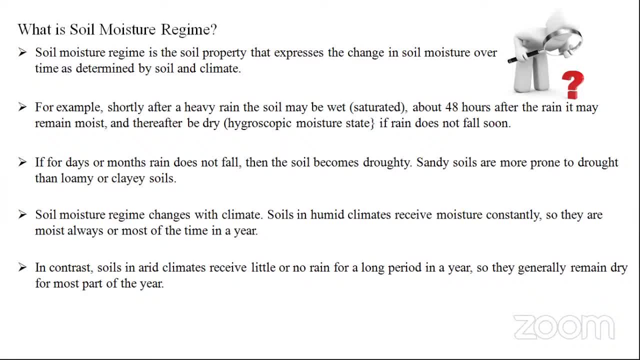 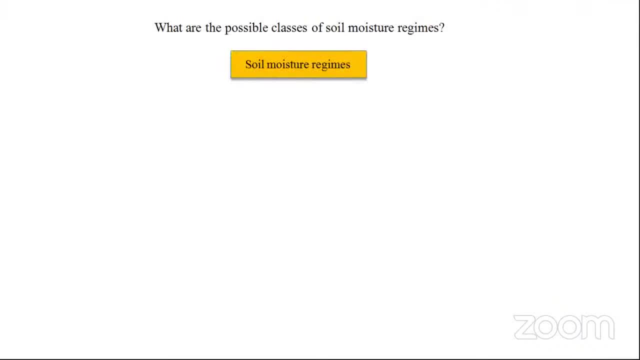 is no rain, nothing, it's completely airy conditions. so that type was that is called one type of soil moisture regime. what are those, what are those terminologies, etc. etc. we will discuss now. so what are the soil moisture regimes? list out students. very first we want to list out the 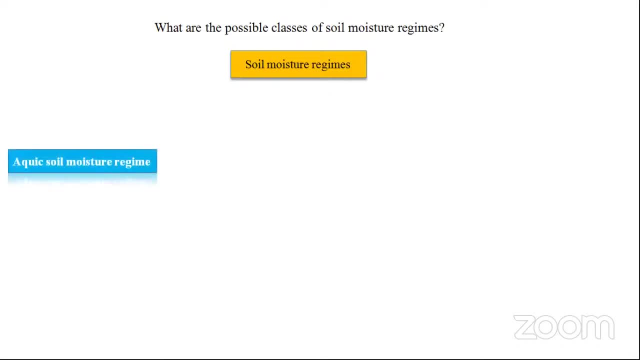 what are the soil martial rhythms? very first one: a quick soil moisture regime. remember a quick. you know there is one famous water bottle company for this, aquafina. just remember like that. okay, a quick soil moisture is the name itself will say what does it mean? what is the moisture condition in? 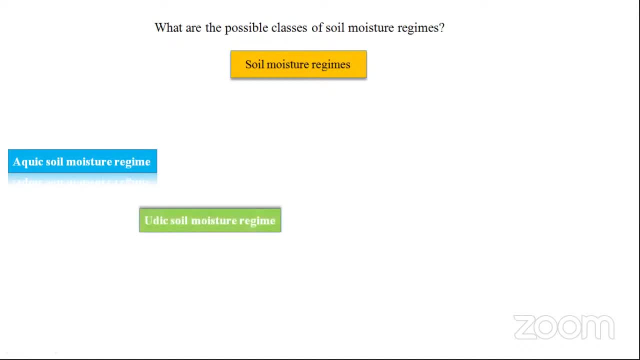 that side and another one is called eudic soil moisture regime- quite interesting- and another one is called erratic soil moisture regimes. i hope you will. you can understand both this very well. opposite to each other: erratic soil- martial regime and another one is called mystic soil. 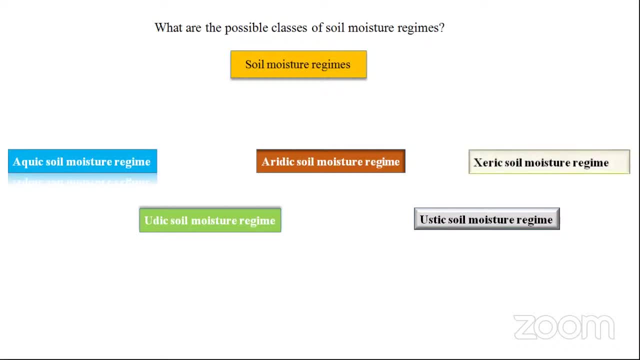 martial regime and next is called zurich soil martial regime. these are the important, these are the- not only, these are the important- soil martialism students. uh, personally, when i was written in jrf exam, even in srf exam also, i have experienced one question from this, both in my career in sr. in jrf i got one question and i 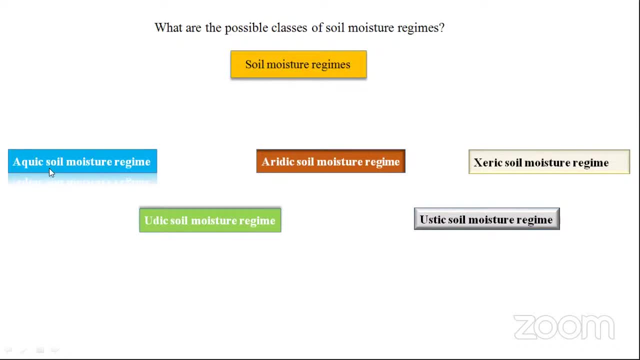 started also. i got one question, so that much importance is there. please be very careful. aquatic soil- martialism. eric soil martialism, xeric soil- martialism, this ludic soil martialism and mystic soil martialism, just to remember. so soil moisture will be going on increasing. 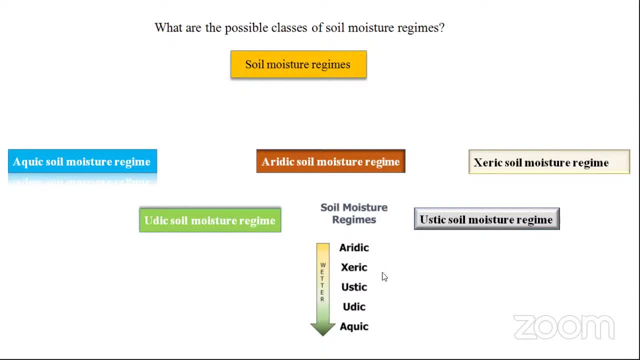 just put, just write note down in your notes like eric, xeric, rustic eric and equity. so when you go it will become very better and better. the moisture condition, this aqua, of course, complete saturation, we will see all those things. so it is not done like this. so these are the soil moisture. 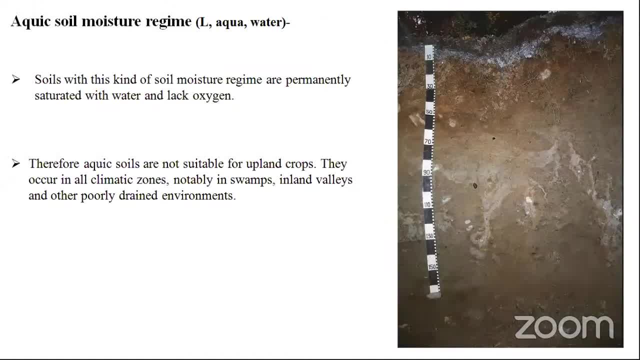 raising. okay, students, aqua means in latin world, aqua water. okay, so in this you can see soil permanently saturated with water. act quick. completely saturated students. there is no oxygen because it is completely saturation conditions, therefore aqua conditions for a plant crops or plant problems, some, where the crops of our crops are saturated because in 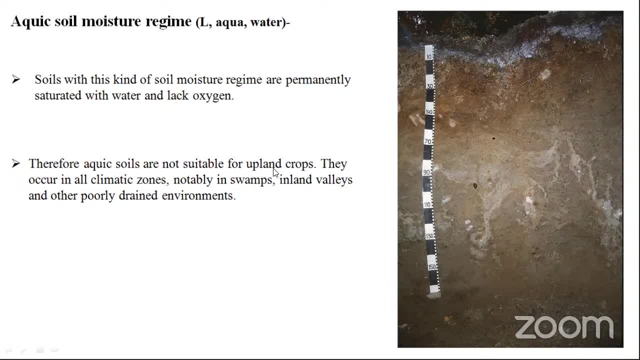 the soils where there is complete moisture will be there. so can we grow vegetables in the style students? no, sir, why? why, rami, please, quite welcome, because you know everybody, because your srf, should you have some experience? jrf students, you answer. why can you grow articles around vegetable crops like tomato, brinjal, all solanaceous crops, i think one student. 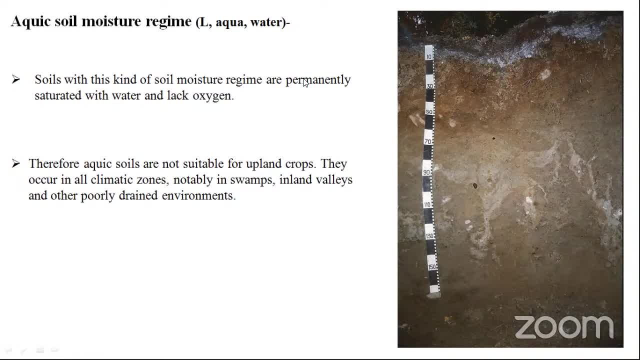 is from this thing, articles, university. why can we grow this here? the condition is, like these students: completely saturation. there will be complete water will be there. entire soil was completely saturated. there is no oxygen and also i'm saying that these are not suitable for upland crops. they are. they occur in. almost this occur in. 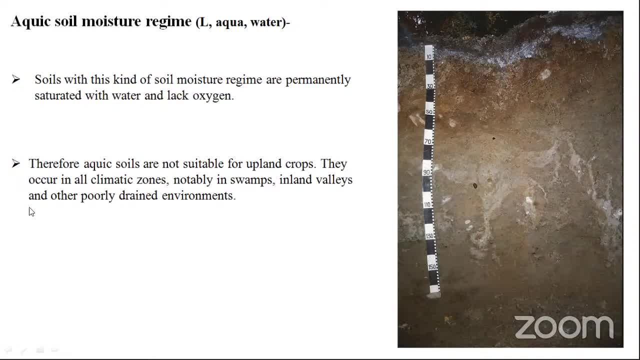 all climatic zones not available swamps. in england valleys, neither poorly drained, end run where the drainage was there is not properly managed. you can see this type of soil, this called soil. moisture is activities. completely saturated means water. the very famous water bottle company called aquafina, just remember with that, okay, can you say, can you grow for some? you know these. 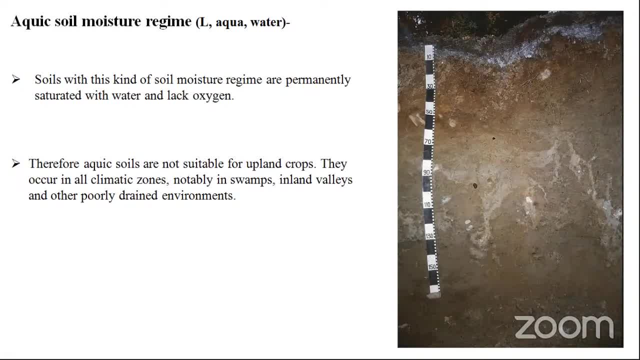 vegetables. can anybody answer students, you will get this type of questions only. you will ask me applied questions. don't think every question will be directly. icr has become very strict nowadays. they're asking very tough questions. please be careful. please answer. this is a very applied question. the condition is like this: 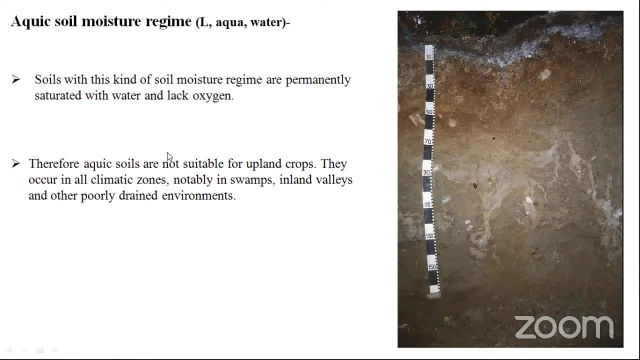 the soil comes under the aqua, aquatic soil moisture resin. can we grow vegetable crops? options are like this: yes, we can grow, no problem. second one is: no is very, very harmful. three: uh, sometimes we can grow, sometimes we not we grow. four: they're not the elbow, they. they ask like this: 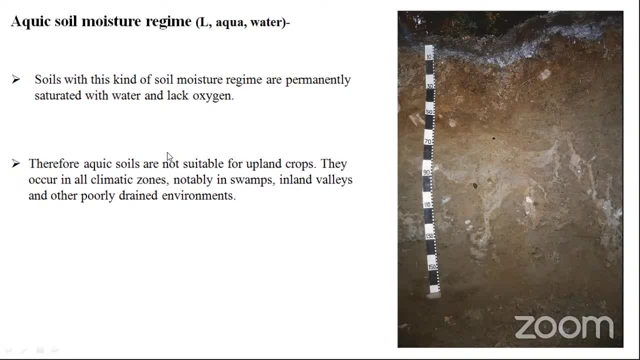 example. can anybody answer okay, i will say answer. you will say reason: okay, no, you cannot grow the vegetable crops in this type of saturation: water condition, aquatic soil, moisture, resin conditions- why? what is the reason? discuss, my god, are you following my class? so reducer conditions, toxic substances are okay okay. okay, you are talking about chemistry, okay. 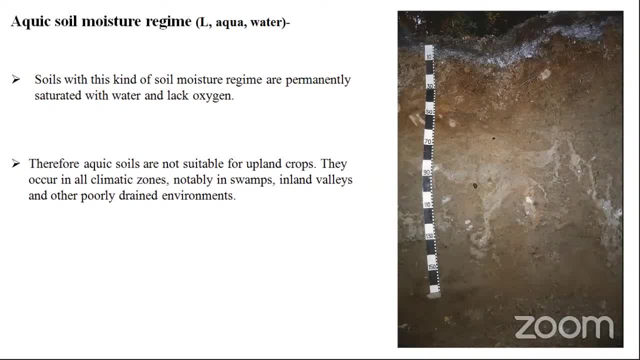 submerging conditions. this completely toxic conditions will be there, so we can't. we can't grow, for why? okay, that means uh, if there is toxic conditions, why we are growing paddy in submerging conditions? that is one point, is there? now you are saying that. 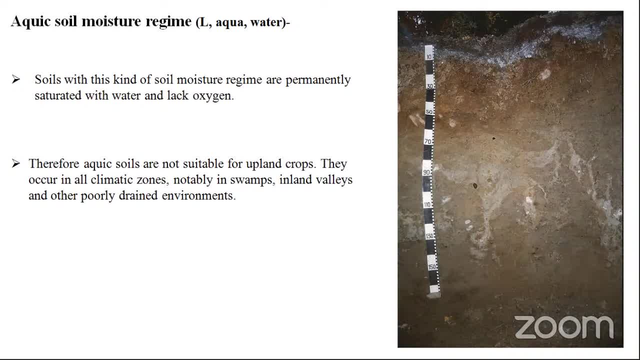 so in submerging conditions, all the nutrients will be reduced. sometimes there will be some toxic materials also will be there because there is lack of oxygen. okay, that's why we can't grow vegetables. you're particularly saying. this is actually. this is one point. is that a reducer? 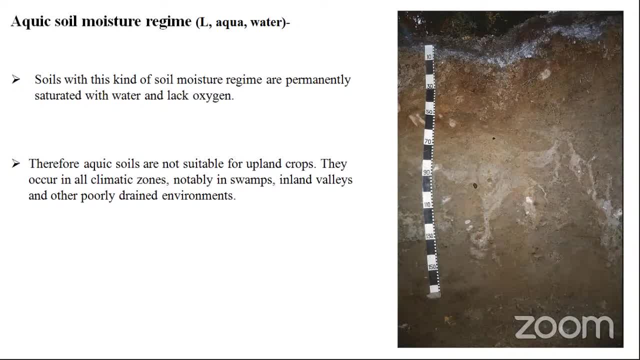 condition, but we are growing paddy now in submerging conditions. can i, can you discuss? come on? the questions will be like these: students those days, the days were changed, asking directly to the students: how can i grow vegetables? questions: what is the if the silica was washed out? iron oxides were left out in this alarm it. 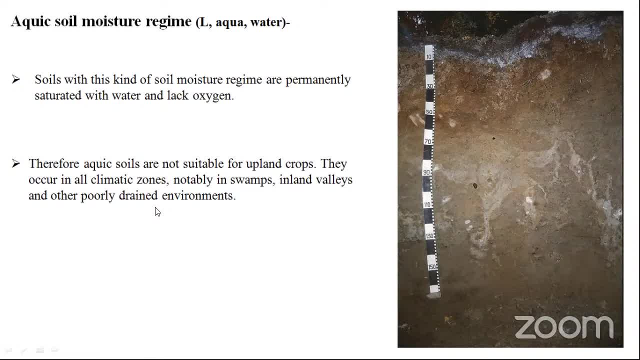 is called dash lateralization. that type of questions were gone, they were expired. they were very old, old-fashioned ideas. nowadays, everything we need, we need a very applied manner. can anybody answer why? you know what is a peculiar condition of horticulture crops? you know students, especially in andhra pradesh. 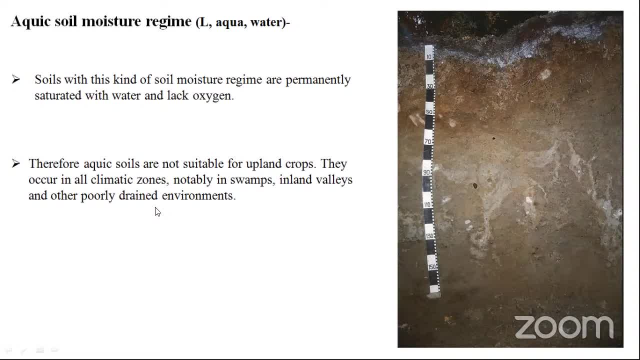 most of the vegetables are grown in chittoor and kadapa. kadapa can grow for banana and anantapuram we can grow some tomatoes. they are growing very well. i'm coming to in tamilnadu conditions, madurai. i think madurai is famous for its flowers and vegetables, theni, i think, then even madurai also. 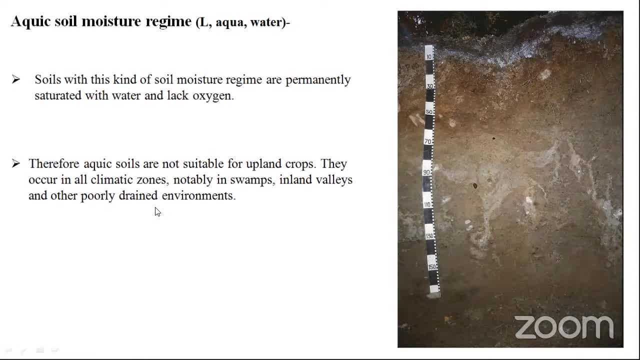 we can expect some vegetables. so why- okay, anyone can answer, i mean you can answer if you know. means destination also see ね- can not be grown. yeah, this one point is there, but overall, students with horticulture crops in suburban conditions cannot be grown. most of the horticultural production can not be grown. most of the article. better than that, a lot of them will, will grow, can we can grow if good enough to need. 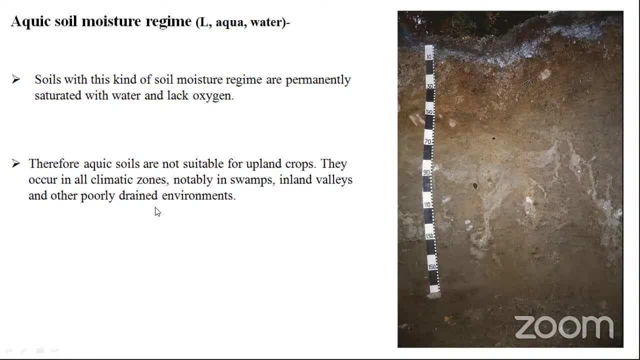 crops, you see whether it's vegetables. most of them are in plantation crops, also in submerged conditions. you can't export any crop because- because the submerging conditions will be there, root system was not properly grown, but paddy can be, can be survival. why paddy can survive in submerged conditions? what is the reason? 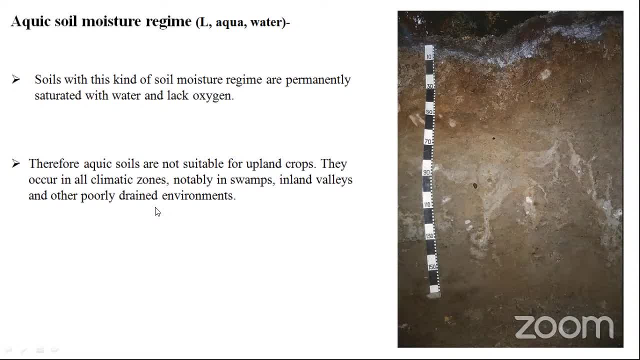 okay, come on, come on discussion. you need a lot of discussions. this is, this is the question, this is the class should be like this. what is the reason why paddy can grow on? because, well, the answer is right, what she said right: vegetables cannot be grown in saturation. 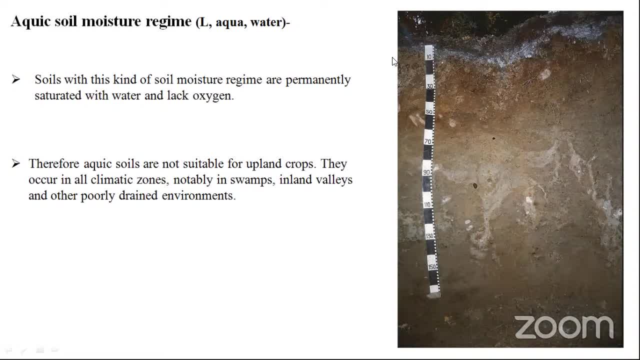 condition. why? because the root system is like that. there is no, there will be oxen was completely seized off. there is no oxen. that way, vegetables cannot be grown in aqua soil moisturizing, but paddy can be grown in submerged conditions. what is the reason? can anybody say? 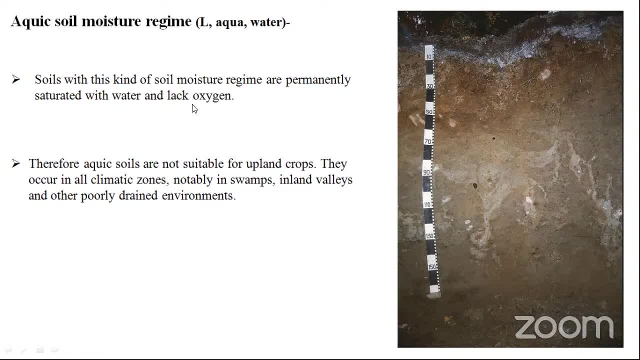 what ma? presence of air and cameras? yeah, there is a. yeah, there is. yeah, there is some. actually the there is special mechanism in paddy. the respiration, the oxen will flow from the sacks, that there is a particular system will be there. that's in physiology. we will read all these things. 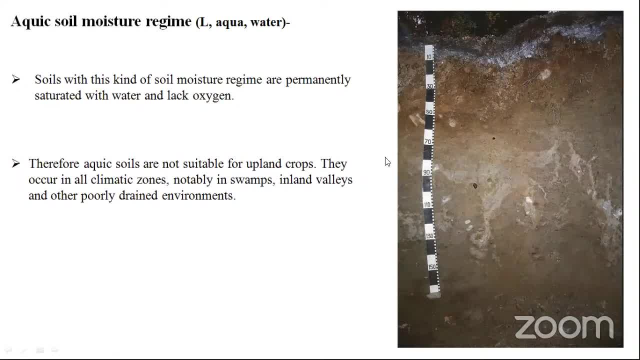 from that it will go, the oxygen will respite. that is why. that's why paddy can can grow in submerged condition. even paddy can grow in some semi-arid drought conditions also can be grown in some semi-arid drought conditions. also can be grown in some semi-arid drought conditions. 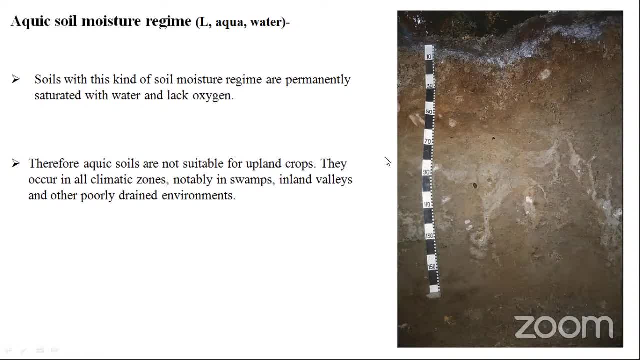 try to apply your knowledge. don't you know? don't, don't mug up. those days were gone. everything was changing nowadays. so anyhow, oh, we have, we have, we have side, we have gone to somewhere with the class. anyhow, this is regarding the aquatic soil. at quick soil moisturizing, epic means completely. 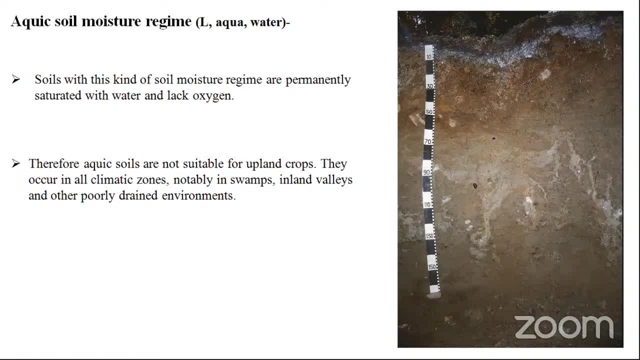 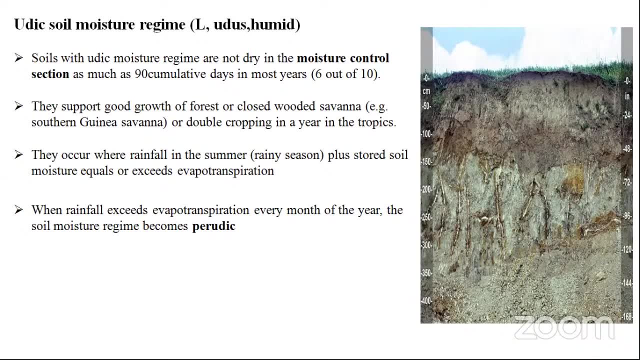 saturated. okay, student, this is regarding the academic soil conditions. i'm coming to the unique students. unique makes humid conditions, mostly in humid conditions we can see mostly um in. unique also may not drain moisture control conditions up to even 90, up to cumulative 90 days, up to 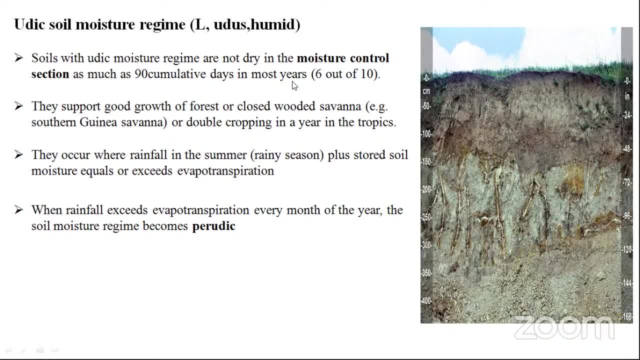 up to for 10 days, six, six days. it will be in moisture condition, only it will be. it will have some sort of moisture will be there, there in uniquely. that is the opposite. the previous layer is opposite. you can complete submergence, but you can here, you can see some sort of 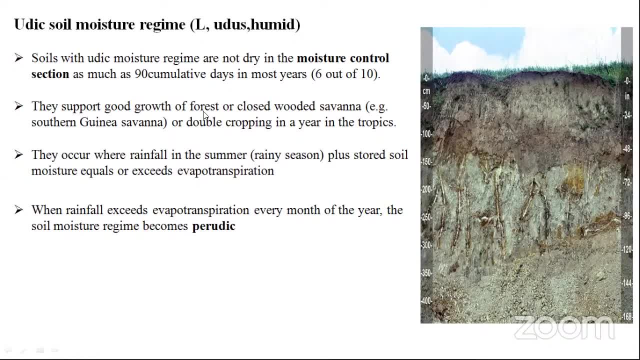 moisture condition. condition is there. so that is why here we can grow some forest crops, some wooding crops, even we can grow for double or double cropping areas. if this condition is prevailing, we can grow for double cropping areas, we can grow for double cropping areas, we can grow two crops, two crops for itself. most this type of- we can see- valley conditions. you can. 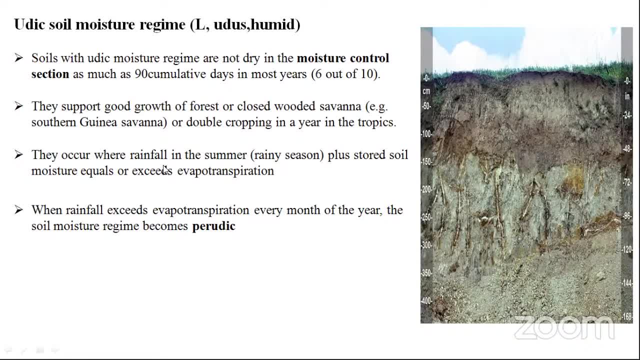 see, i mean some riverside, all the already you can see they are. they occur rainfall in summer mostly. we can get somewhere also let's store this soil, moisture equals or excess, the vapor transmission okay. so so mostly in summer also they will get some sort of, uh, some sort of rainfall store. 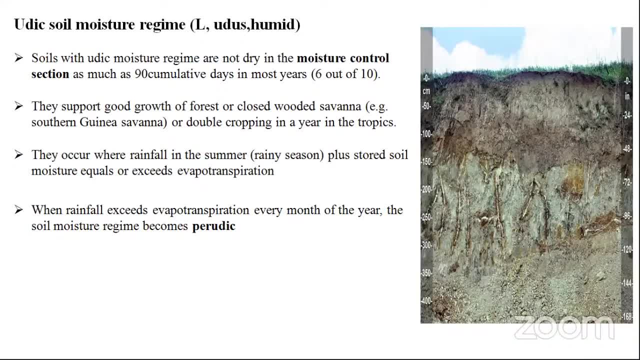 moisture equals or sometimes it will show it with the soils, will store moisture equal to vehicle transpiration or sometimes even exceeds the vapor transportation also. so that's the conditions. if the condition is like that, if the rainfall excess, the evapotranspiration, even months of year there is a heavy rainfall than 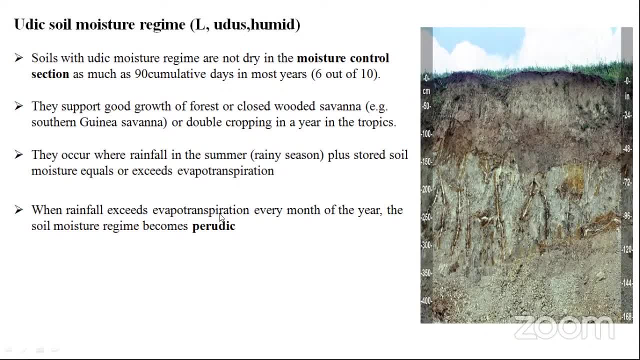 the evapotranspiration so that soil moisture can be called pre-dig conditions. this is the condition stress. it means it's somewhat moisture. you can see this is a moisture control section. after 90 days it will be so mostly we can grow for uh forest crops, we can grow some sort of double. 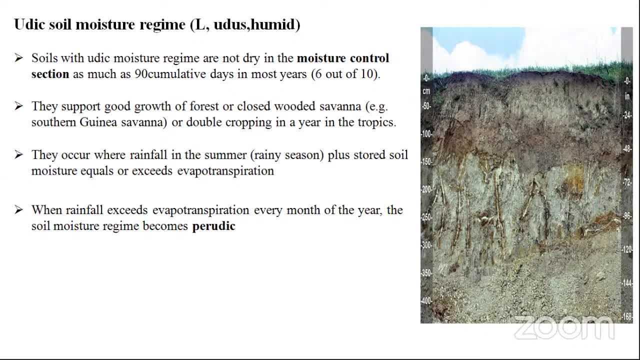 cropping we can. we can go for two crops, two cropping a season. we can grow if the condition, the rainfall exists, the evapotranspiration every month, every month, is it was repeating more rainfall, so that condition is called the pre-eudic conditions. okay, students, remember this is. 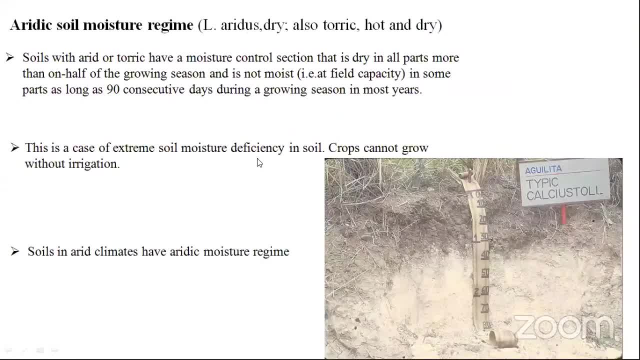 called the eudic soil moisture resin. this is regarding this and coming to the erratic conditions, you know there is no need to explain it because the name itself is explaining: erratic means dry, also toric hot, and dry erratic means hot. so here you can see, students is completely dry in all. 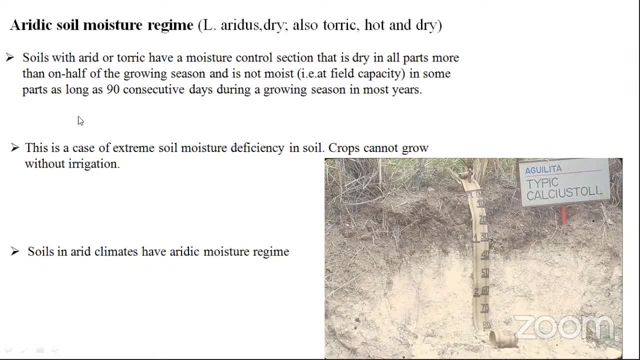 parts almost it is completely dry in all parts in growing season is not moisture. so most, in some parts of 90 consecutive days, it will be completely dry conditions. so in this type of arid soil- arid soil moisture is- we can expect only complete- uh, complete- dry conditions. so in this type of 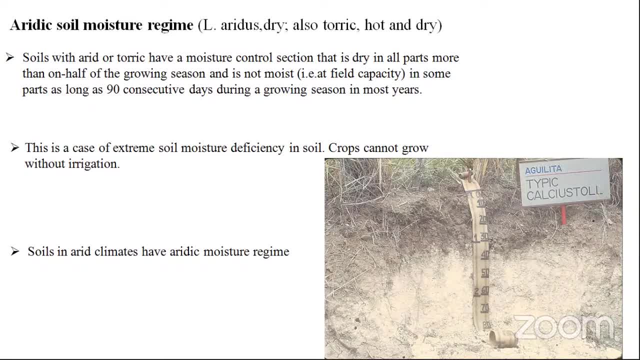 situation. we cannot grow crops, so without irrigation- i mean without irrigation- you can't expect any. any cropping is the soil in arid climatic, having arid moisture conditions. so definitely, please remember, students, sometimes the question will be very tricky. you should be very confident in your answer. you see, arid means dry condition. 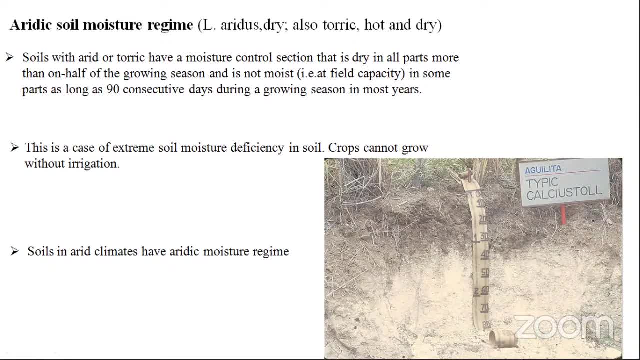 arid is also. you know, they will, they will, they will come by, compile all these things. sometimes they will compile the if, the, if, the. if the condition is like this, if there is no rainfall from years to the years together and crops cannot be grown without, without any proper irrigation, 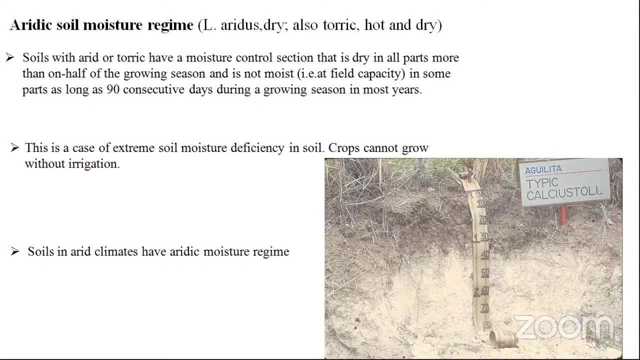 without any proper, proper irrigation, there is no more. there is no more moisture. what kind of soil moisture is will prevail? the questions may be like this: it will be applied questions. that is called the erratic soil moisture. so you should go like this. okay, students, be confident and be applied manner. the community is called. 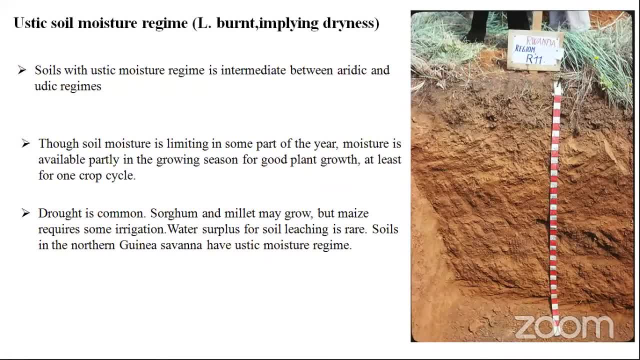 strict moisture reason: so burn or imply implying dryness. no, implying dryness means it is somewhat characteristics between the erratic and ludic students. it will be very intermediate. it will be intermediate between erratic and ludic in which? so what is the first? oil, moisture or somewhat. 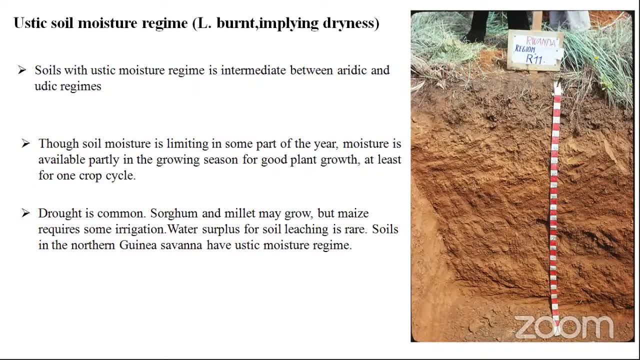 limiting some part of here, it will be very limited. moisture is available by growing season for good some. we can grow some, some sort of cropping growth season for a good plant, at least for one crop, yes. so here the moisture conditions are somewhat like this. so mostly this is what stream this type of 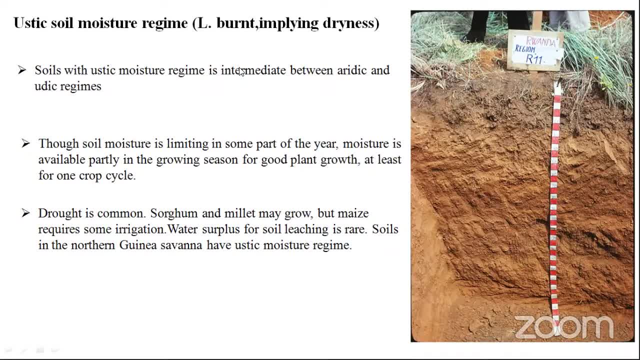 soil moisture regime prevailing in the southern coastline, especially in precaution district, you can see this type of situation. this type of crops are. this type of conditions are prevalent. we can hardly we can grow for one crop, one crop one season. we can mostly. what type of crops we can? 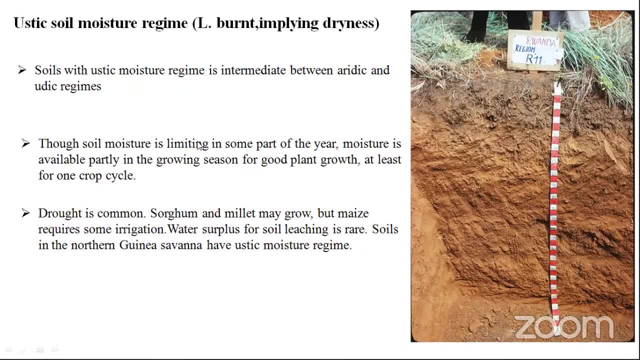 grow in this type of very light moisture condition, this type of stick moisture situation. we can grow sorghum, millet, millets may grow, as i said previously i said, and maize requires some irrigation. you want to grow maize means we can grow if there is any water. irrigation supply is there, means we. 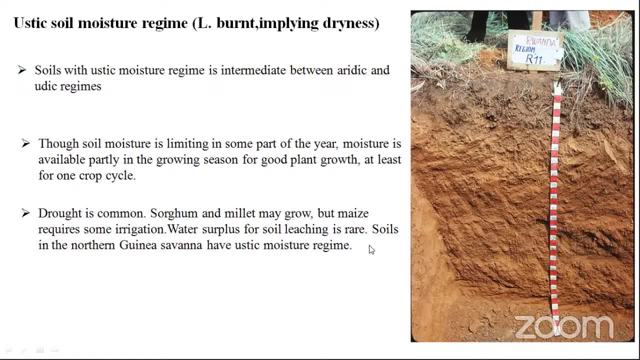 can grow for maize and water supplies and leaching is very rare, students, because the moisture is very, very lightly available. and where, where is the chance for leaching so soils are? because it is not savannah is we can see this type of stick soil moisture, so the moisture is very limited. 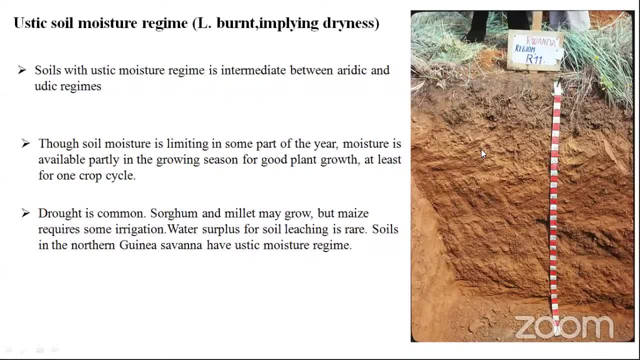 moisture will be, the stress and the dryness also will be there, but moisture was very less, you know. but we can grow one crop. we can grow one crop in this type of stick soil, martialism. what kind of we can grow? we can go sorghum, millets may grow. the question is: remember, remember the concept. 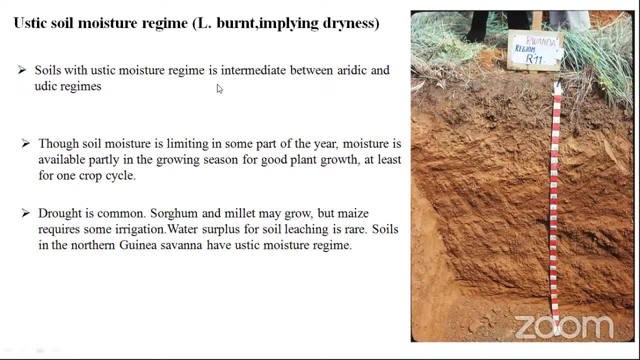 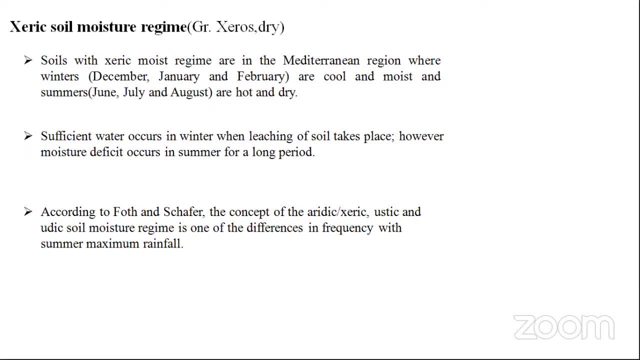 concept and idea that is very important. this is regarding the stick soil moisture. finally, ziric moisture- like completely dry, this is also dry. the soils with ziric moisturizing are mostly we can see in mediterranean reasons, where the winters, especially december, january, february. 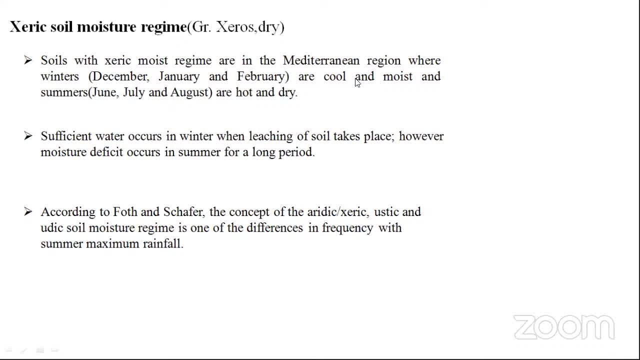 you just see this uh climatic and say where it's suitable, and cool, moisture conditions like june, july, august monsoons. this is, i think this is uh. this is uh the point in time where georgetown has managed to build a lot of material. 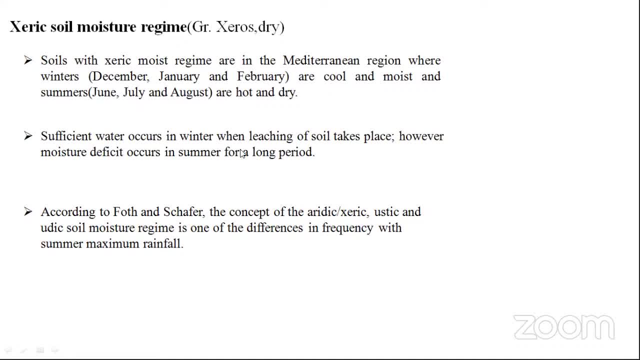 but it is not a boundary area. much of this is part of one of the huge reasons why we can get the parts of siri, which is sunflowers. so sunflowers are one of the main resources in the south west, so in some places we can get some of these uh months. we can get the southwest. 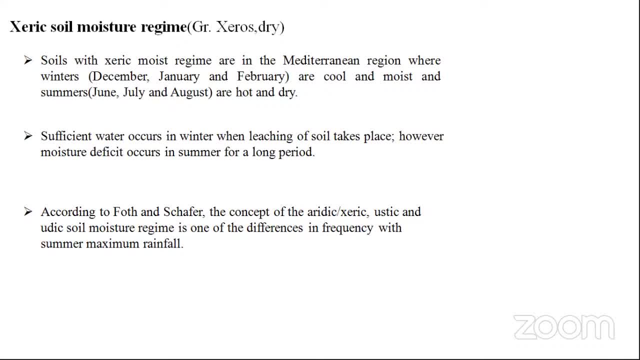 and here we can get the northeast masses mostly under appreciation. most of the place was influenced by this, but most of the tamil nadu was influenced by the northeast monsters, if i'm correct. so so of whenever the water is available, there will be plenty of water leads to the moisture washout. 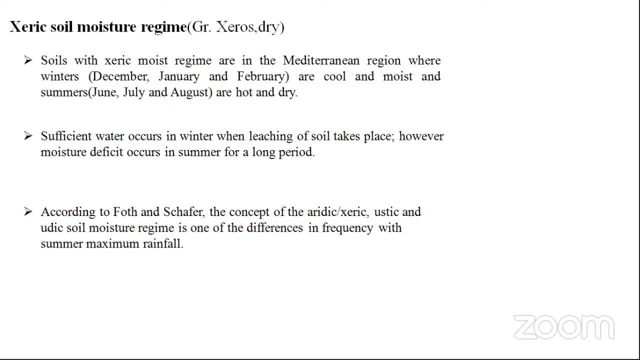 but in summer, completely drought conditions. this is the condition in zeric conditions and if i want to say in some informal language- in telugu there is a one word. it means means we get enough friends, which is now, which is now enough, more water will come on our history. that means no, there is no water, complete dry. so situations will be like this: 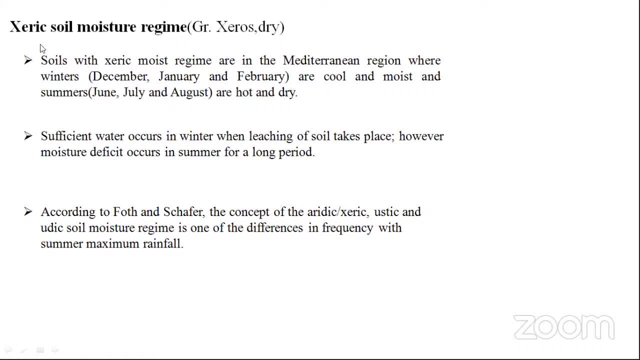 there will be, sometimes it will be more rains, sometimes very less strength. so here also situations like the xeric soil moisture conditions. mostly there are two people. fourth, and the snap forward concept of erratic and xeric and a stick anodic soil machine is one of the different in. 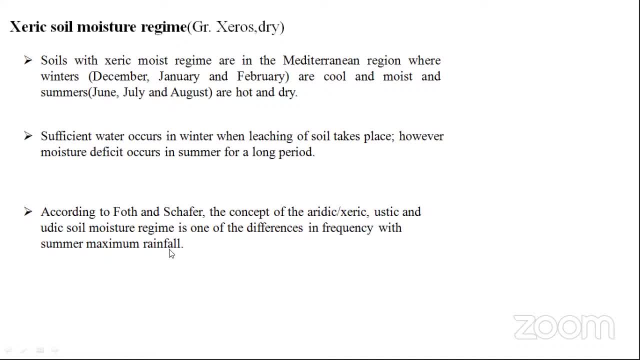 frequently with summer maximum maximum rainfall. so mostly this type of uh soil moisture regimes we can see only depend upon the climatic and soil moisture, rainfall etc. based on these two, summer and rainfall, will decide this type of conditions for xeric moisture conditions most heard. sorry, or you will already be aware, um, you have a quick q a air. 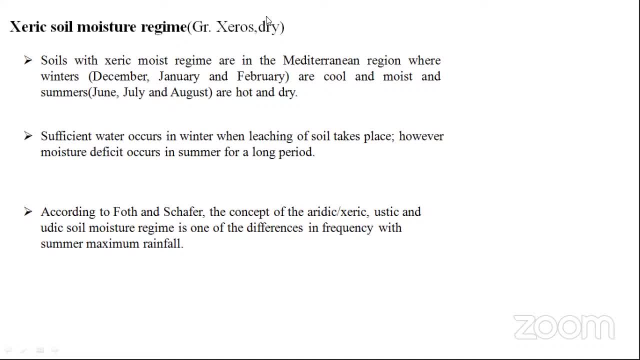 do you have any idea regarding your area? can you give any? i can you give any example for this type of xeric moisture situation in the area in your particular state? okay, answer as usual anyway. so this is regarding the soil moisture regime. okay, so what is the? 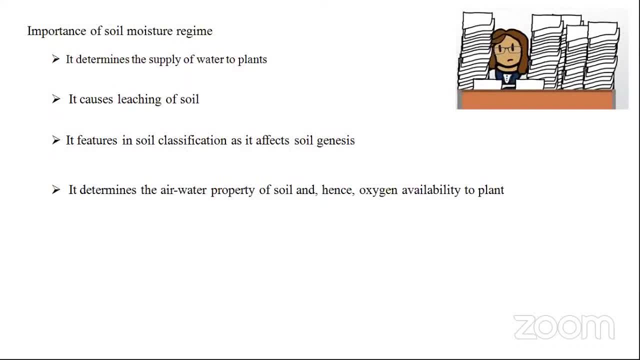 important strengths why we are reading the soil moisture regime, which is thatDPRES Platform A‐ washout has become extremely important, as i mentioned above here, as we suddenly threw some perish with homepage. mainly determine the supply of water to the plants. very first. it's determined the irrigation part. 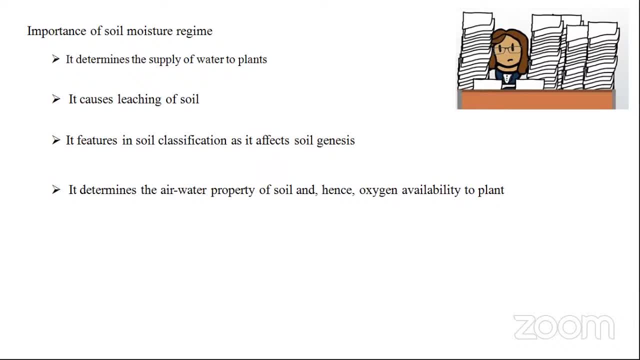 supply of water and it causes the leaching of soils, especially that even we will deal with that one also. so it is the future in the soil classification, as i said in very earlier soil classification, and it also affects the genesis which we have discussed in the very first lecture. 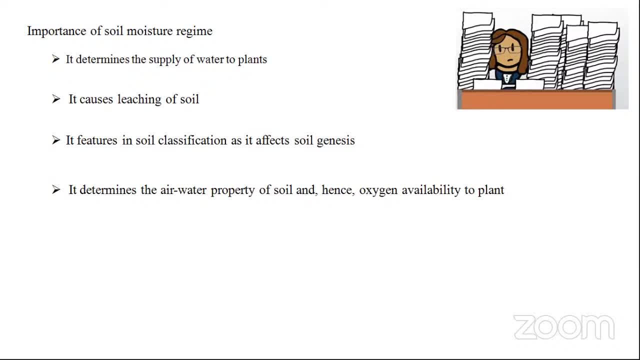 it determined by the air water property of the soil. hence oxygen availability. is the plan? mostly oxygen conditions, especially that way what we have discussed so far, the oxygen supplies it will determine. so this is a major importance for the soil moisture. is that we have to discuss? okay? 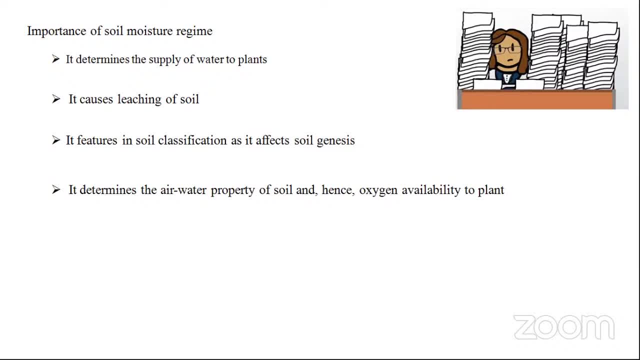 students, this is. this is up to the soil marshals. if you have any doubts in soil marshals, we can discuss. any doubt, students, there is no doubt. we will go for temperature regime. any doubts in soil moisture regime? no, sir, actually no. no, thank you anyway, we will see the next. oh this. 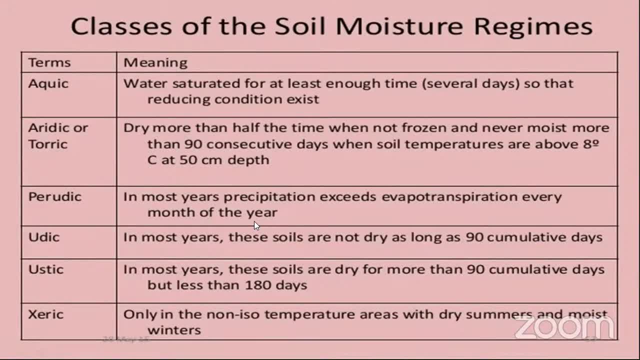 is the key point. stress, this is almost uh. whatever i explained in the previous slides i given in one line. this is one line word. you can uh see this whenever you're watching youtube: uh, repeatedly in this channel, this class. just pause it and read these lines. okay, the same thing. same thing, which. 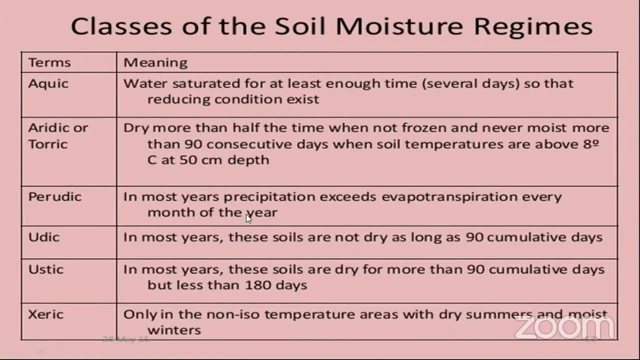 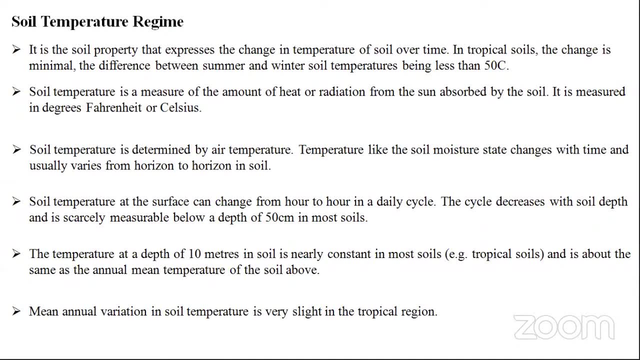 i have repeated is because i put it in a single line, just for your understanding. okay, students, okay, the soil moisture is in soil temperature regime. so, students, mostly, this temperature was completely different. this temperature is nothing, but we will see the difference in summer and winter temperatures with less than 50 degrees celsius, and we will. we will. 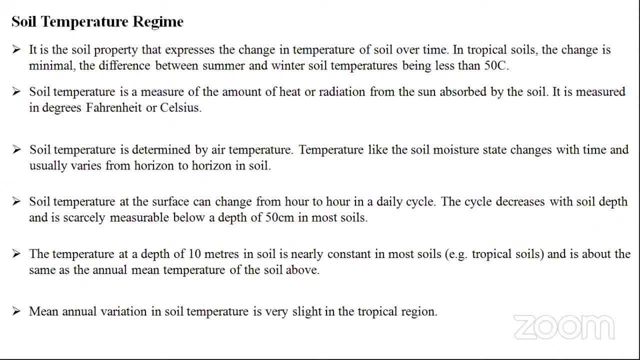 calculate the uh. how much amount of how much heat was received or our radiation was received from the sun. it is measured mostly farm heats or celsius, mostly india. in india we go for the celsius parameters, go for most states. in united states they will go for a parakeet, the indians will. 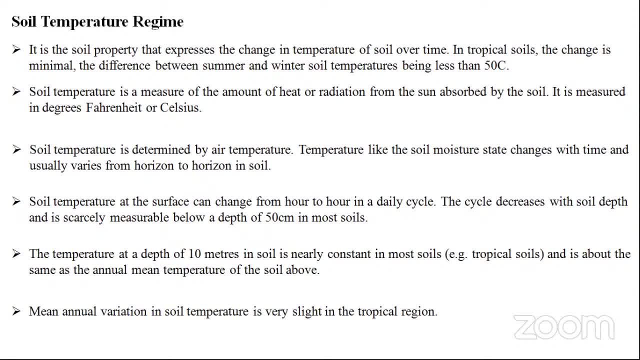 calculate only in celsius. so temperatures- mostly the soil temperature is completely- have completely determined air temperature and also moisture changes. if there is any moisture changes, generally we can. we can expect some temperature changes and also even this. this temperature is completely determined by the bare day conditions. however, 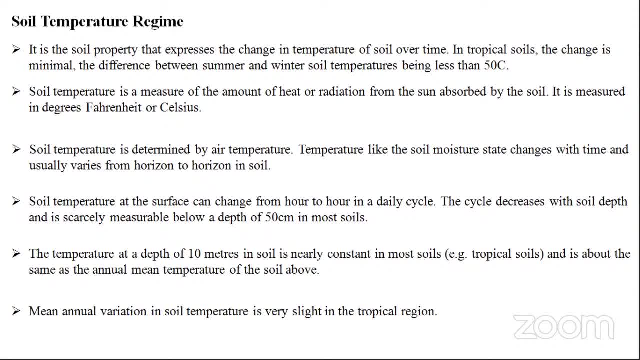 these changes may experience. from hour to hour there will be a change or sometimes we can decide this cycle also daily cycle also we can see some changes. so mostly the temperature, the cycle, mostly the surface changes, mostly decrease how the soil depth is: scarily measured, hardly we will measure. 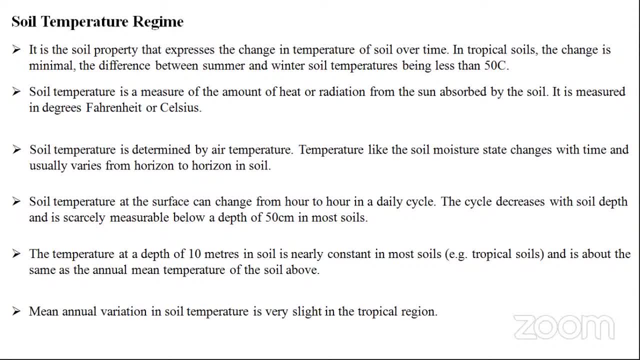 the temperature up to 15- 50 centimeters in the moist in the most soils. most soils will go up to 50 centimeters temperature of the every 10 meters in the sun is nearly consisting of moist soils. the mean annual temperature of the above soil mostly, if we measure this line, is very important. 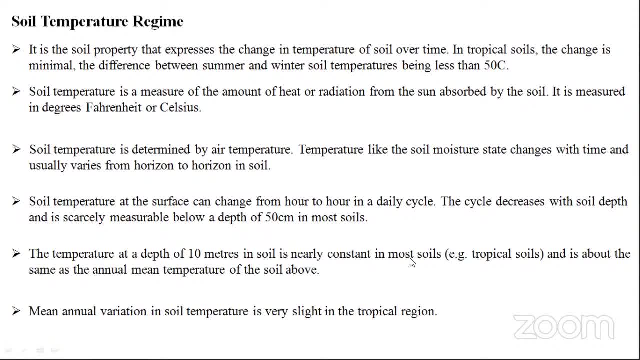 the temperature of the depth of 10 meters in the sun is nearly constant in most of the soils in tropical conditions and is about the same of the annual temperature. so this will give the annual temperature condition for about 10 centimeters. if you measure means it will give the annual. 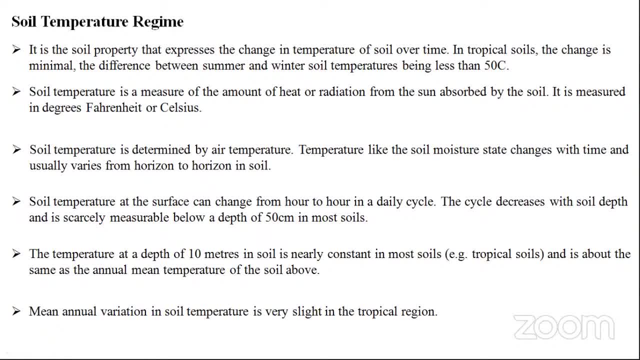 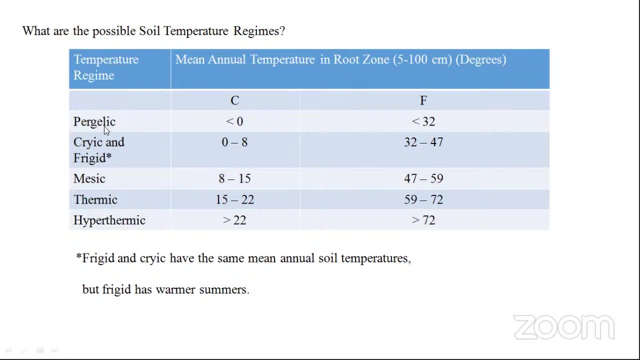 temperature. so mean annual temperature, salt temperature slide. in the tropical regions, most tropical regions, there is. the change of mean annual temperature was very less. which is what? so what are the different possibilities of temperatures, sir? these are the different possibilities. remember, students, you will get one question from this, this thing also, what are those? 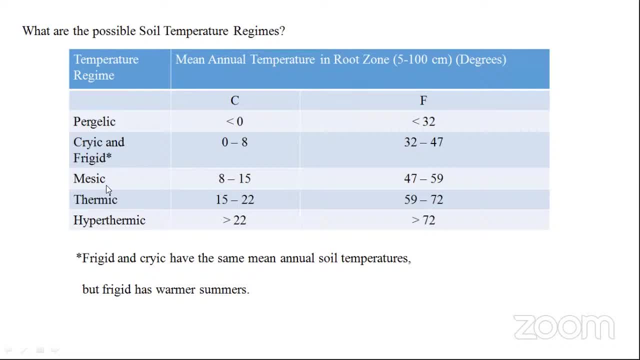 words frigilic crike and frigid music, thermic and hyperthermic. what are the first of all? first of all, utter? you try to spell out these words: frigilic crike and frigid music, thermic and hyperthermic. frigid and crike will have the same moisture, resistance, students, same same. 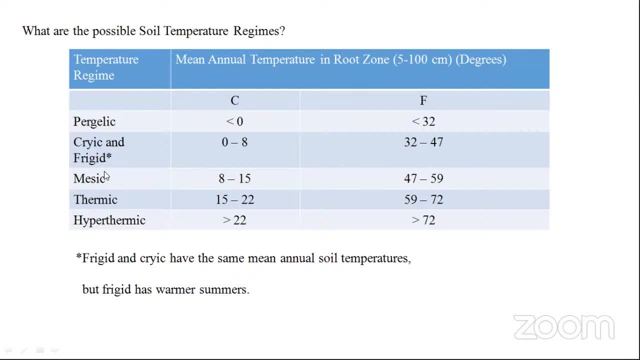 temperature but frigid somewhat will be. a frigid will be somewhat warmer in summers. in summer it will show some slight variations, not that much ways. so very first frigilic. it will be less than zero degree celsius if you want to see in parent heats mostly 32 degree celsius. crike and frigid. 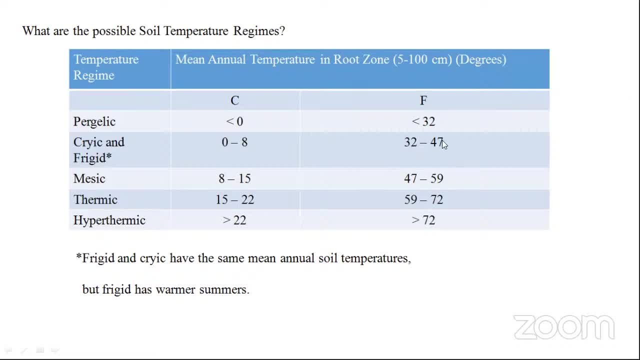 students, mostly in celsius. it will be 0 to 8 in parent heats, 30 to 47 degrees. music: it is around 8 to 15 degrees that we have to convert in parent heat. degrees means 47 to 59. please note down all. 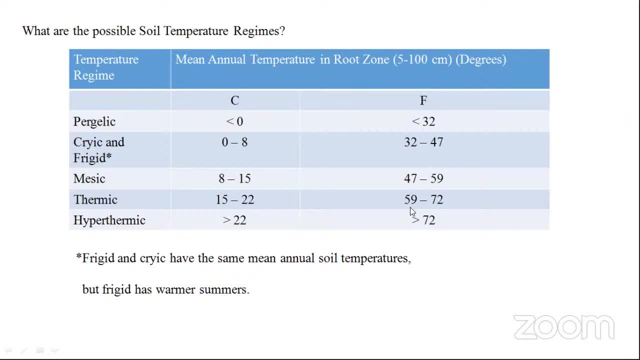 this values: thermic means 15 to 22 in param. heat is 59 to 72. hyperthermic means more than 22. it is more than 72 here in parameters. so these are the different different moisture, these are the different different temperature regimes. so these temperature regimes will play a major role in soil. 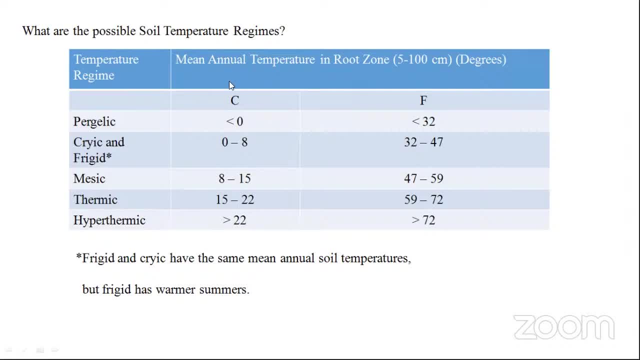 weathering process, what are the different crops we can grow, and it all these are completely depend upon how much moisture are based on moisture availability also. this will be very strong originally. sometimes the frigidly it may go to the music. miss it may come to the fritulic because 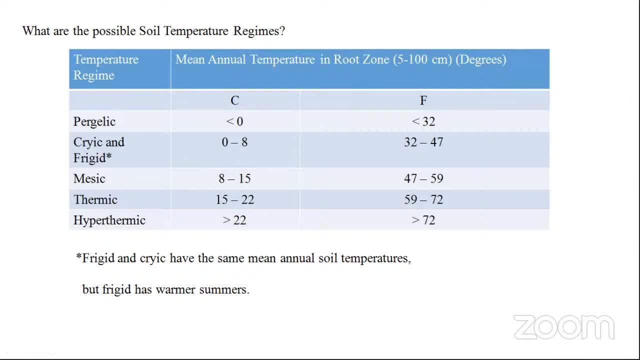 completely depend upon the. there's a precipitation, that is, rainfall. except all this, they have to get. so, regarding the soil temperature, this is any any doubts. regarding the soil temperature is very simple, students. nothing is to expand here any doubts. physics: you will learn many things about soil temperature. this is a 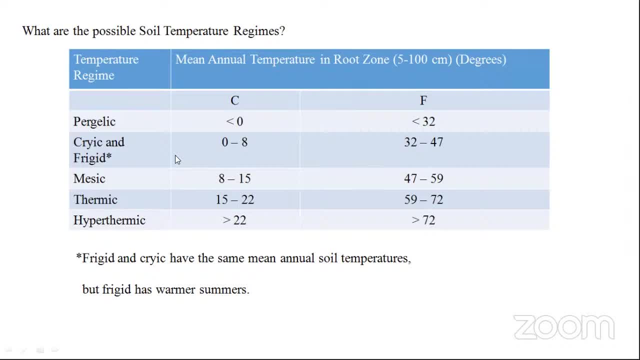 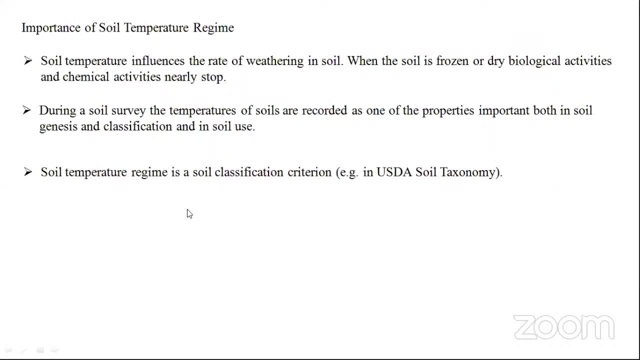 separate chapter. any doubts regarding soil temperature? no doubt, sir, i may expect same dialogue. anyway, thank you. what is the importance out of the important strengths? as i said, it influenced the weathering in the soils, so in frozen or biological activity sunday, and chemical activity really sometimes, this temperature. 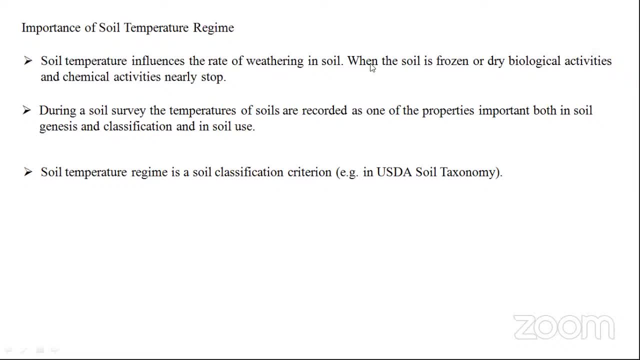 also will place major role in by controlling the biological activity and chemical activity and also during survey- soil survey- the temperature of the soils are recorded as one of the property, both in soil genesis and classification. as i said, we use this temperature both in classification, genesis of the soil, so mostly soil temperatures based on criteria. we take the criteria which 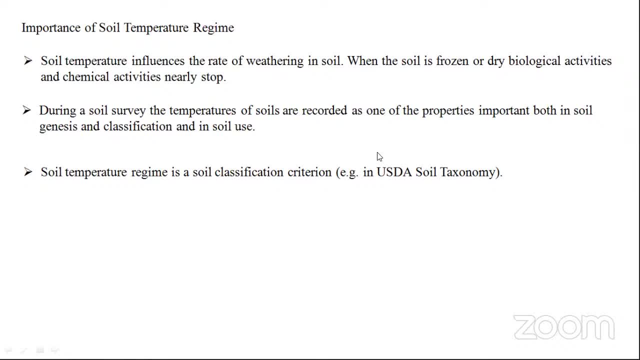 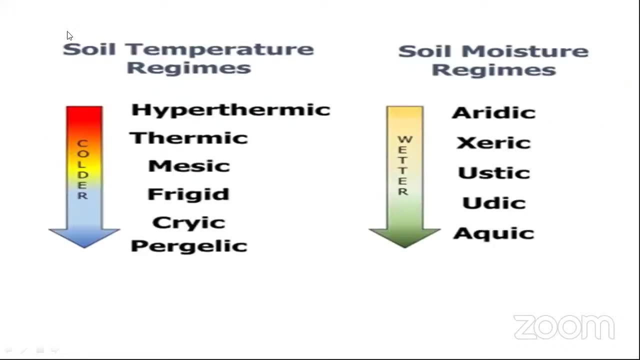 criteria we use. mostly we use whatever we have discussed in previous. another complete taken from the usda soil data axonomy classifications. mostly this was included. this real soil temperature classifications- our soil temperature regime was in, was in- was being collected during the usda soil classification. this is regarding this class and this is the aura view strengths. this is when you go for down and 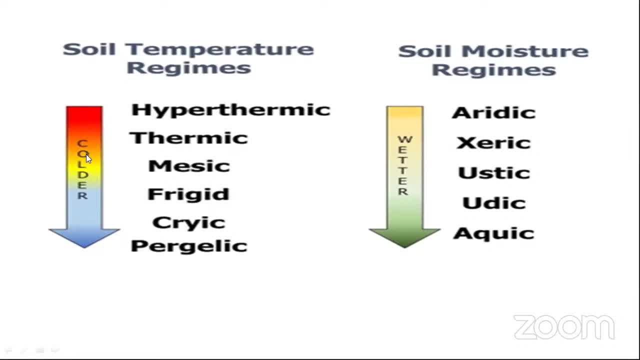 down, the temperature will be reduced. hyperthermic, thermic, mesic, rigid crack and frizzily. you can see if you go very down down this part, just put an arrow and let it down like this. okay, students, the same time soil moisture is, if you go down and other means, erratic, very dry, ziric stick. 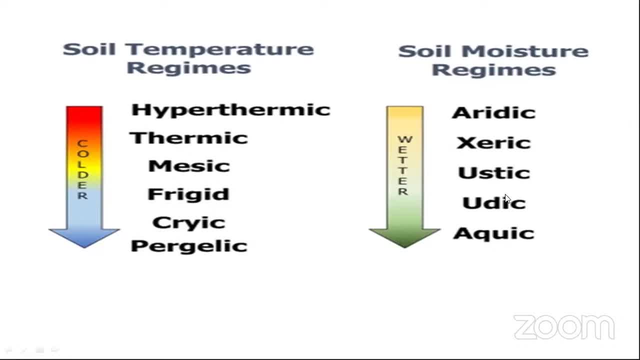 and i could. i could, very completely submerged. here you can. some sort of light moisture will be there. here you can see intermediate between these two ziric. sometimes it will be some much in winter it will be very water. summer we know what erratic, completely dry, you can have.